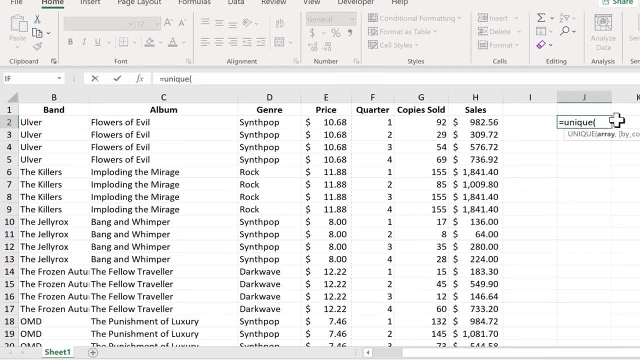 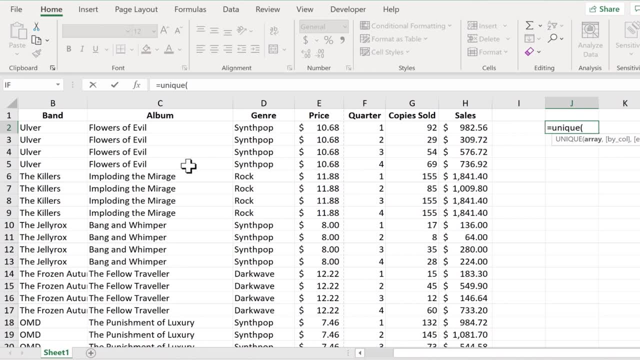 I want- I put in my left parenthesis Now what comes next. Excel is asking for an array. So what's the array that I want Excel to look for unique items in? Well, it's this. It's column B. Now I could select the whole column just by left-clicking on B. You can see what. 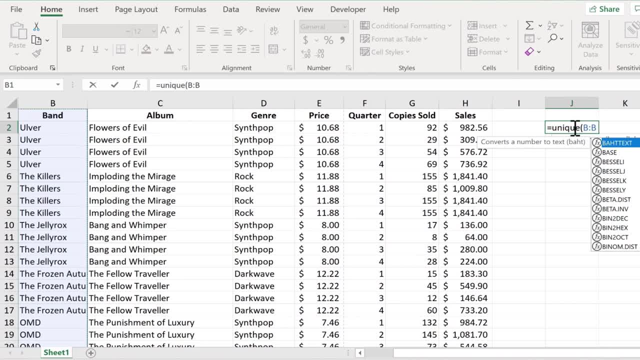 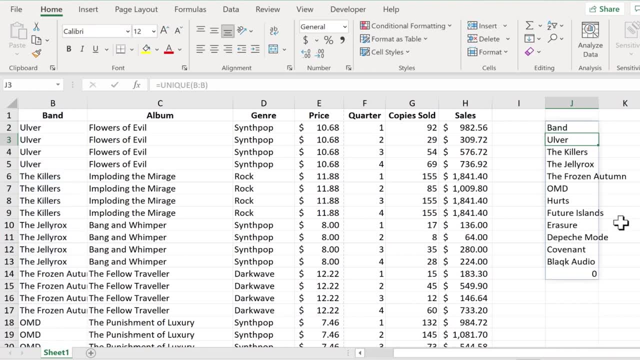 Excel does. It puts in B, colon B, In other words the entire B column. I should put in my right parenthesis. I don't really have to, So I'm going to put in B, colon B. I should put in my left parenthesis. I'll tap enter and you'll notice what it did. It found every. 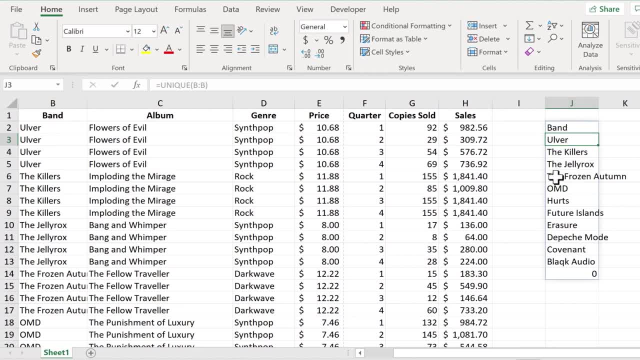 unique word or phrase in that column and reproduced it over here in cell J2.. Now it couldn't fit all of the data in J2, and so it spilled the results. Hopefully you watched my previous video on spilled results in Excel. Now these results are dynamic. We've spilled a dynamic 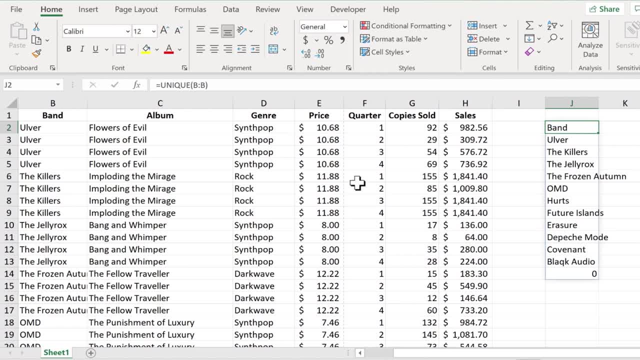 array or range. So now watch what happens if I change the data that that's based upon. For example, let's say I delete the data that's based upon the data that I want to change. If I delete the Jelly Rocks- they're a really fun band. If I remove all references to them, 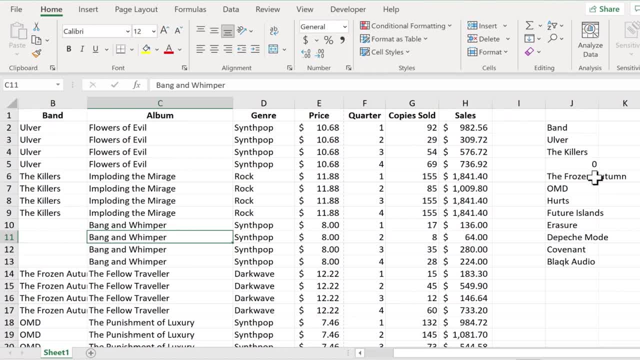 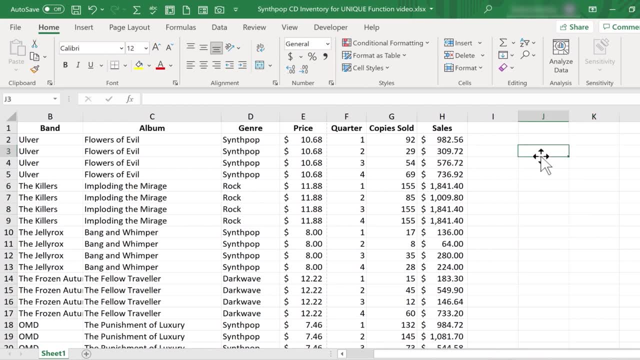 out of the band list, you'll notice that my spilled results change to reflect that. I'm going to undo that. Okay, let's try it again, but this time I want to not only get the bands, but I also want to get the albums. Let's try that. I'll click on J2 and I could click on. 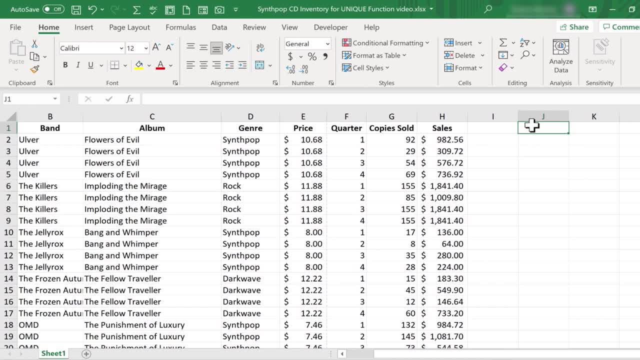 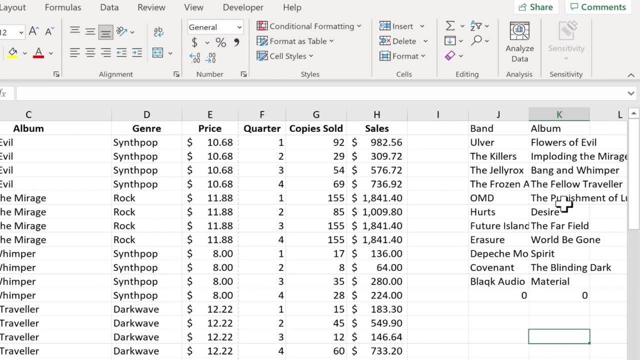 J1, doesn't really matter. Actually, I think I'll go with J1 this time. Equals unique: left parenthesis, Drag from B to C, right parenthesis, tap enter and look at the spilled results. It spilled both the album and the band, but only the ones that are unique. So take a look at. 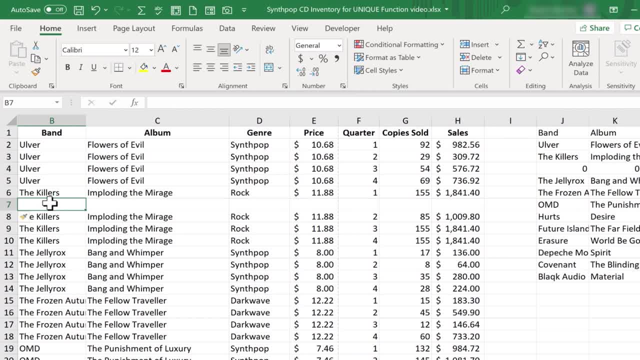 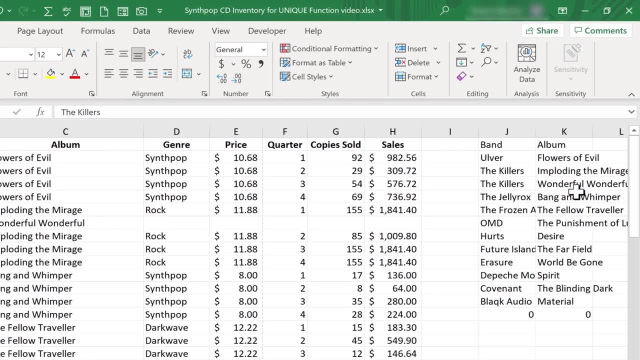 what happens if I insert another record, Let's say The Killers, Wonderful, wonderful. I tap enter. Look what happened to my dynamic range or dynamic array: The spilled results change to reflect what I've added. Now you might say: but wait, the band The Killers is not. 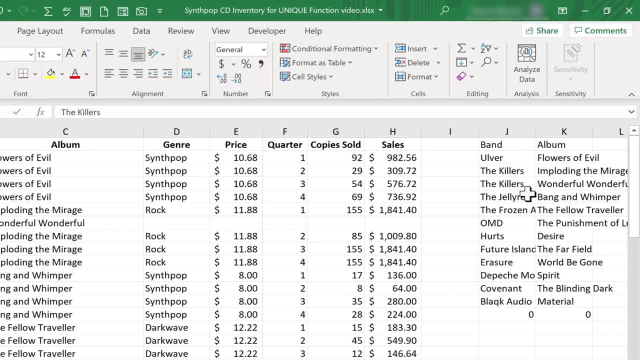 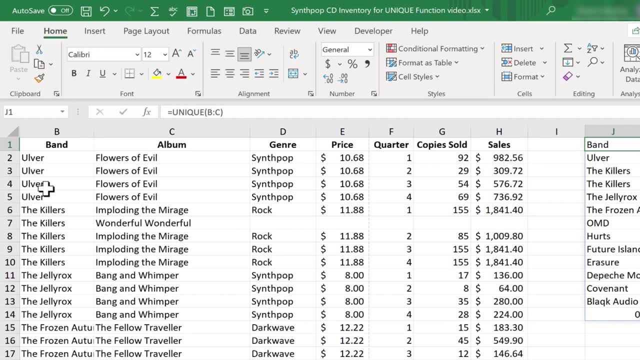 unique from the band The Killers. Well, that's true, but in my formula I said I wanted what's unique in columns B and C. So it takes into account the data in B and the data in C to decide what is unique and what is not. So, because the band and album together are unique. 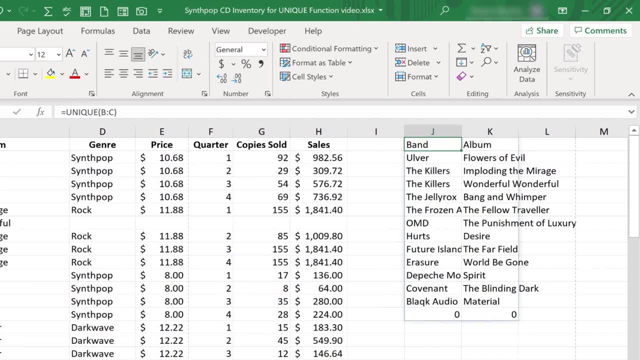 it is listed here in my results. Okay, the next thing I'd like to try is I would like to not only filter out the things that are not unique, but I also want to sort the results in the band name. Let's see if we can do that. So I'll click on J1.. I'll delete the. 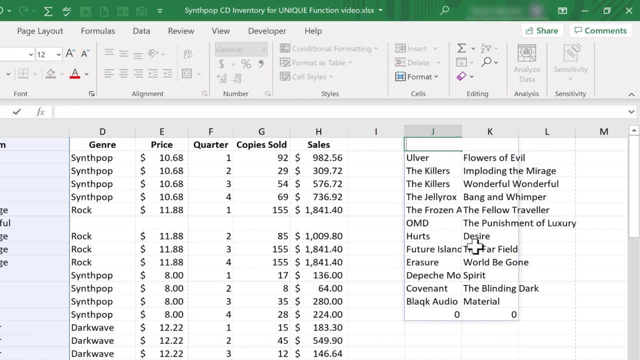 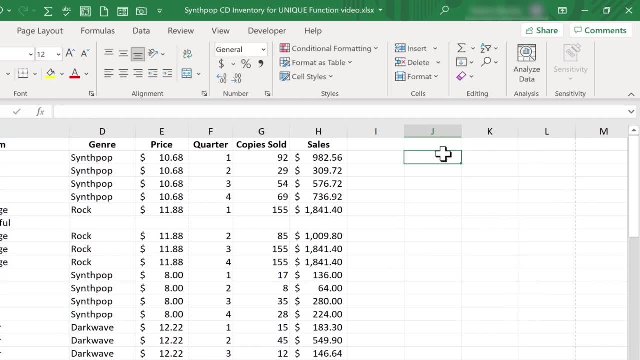 contents of that cell. And, as you know, all of this spilled data is generated based on the formula in J1. So when I delete that it gets rid of all the spilled data. So here in J1, this time I'll type equals- unique left parenthesis and then I'll type in sort. 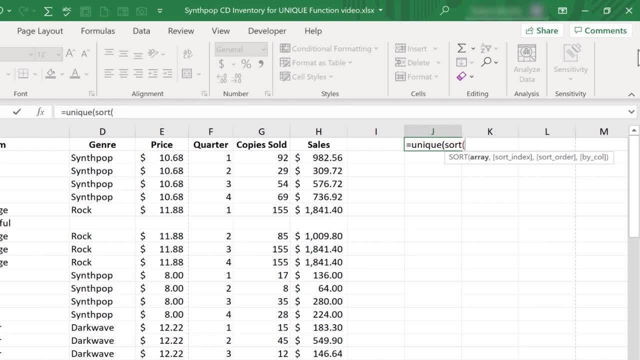 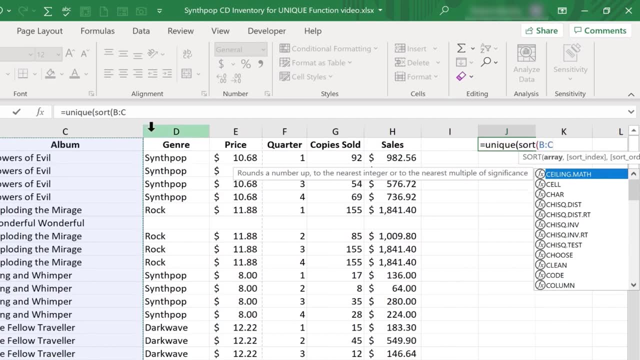 Sort is another dynamic array function. Left parenthesis and then I'll go over and choose B and C. Let's take a look at my formula. so far, And often it's best to look in the formula bar for this. So let's look up there. At this point I'm going to put a right parenthesis. 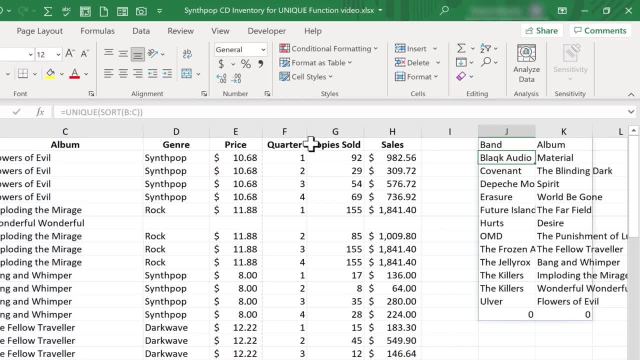 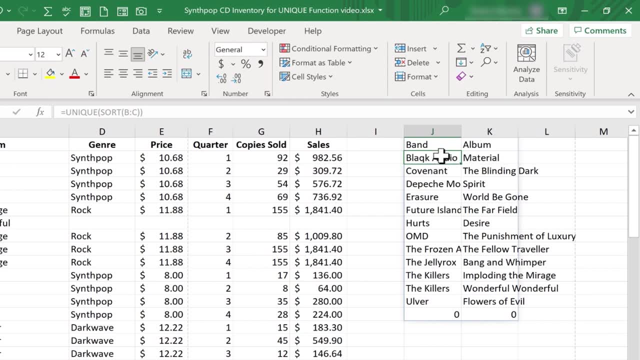 and then another right parenthesis: tap, enter on the keyboard and just take a look at those results here at the right. Not only did it produce the unique albums together with the bands, but they're all alphabetized based on the band name. Now it's also possible to: 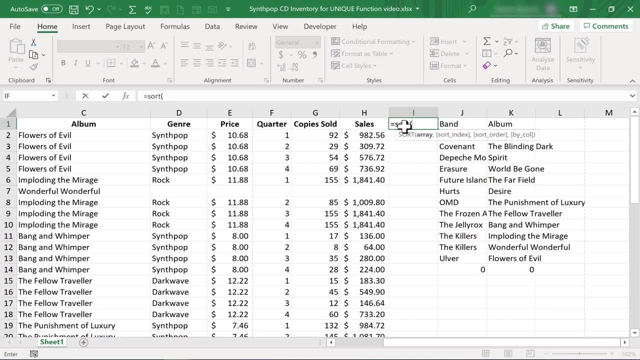 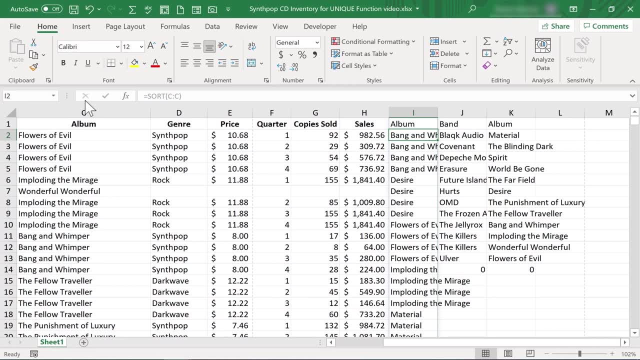 do a sort just by typing equals, sort, left parenthesis and picking a range in this column, tapping enter. So you can just use the sort function to sort any range and spill the results below and sometimes to the right. So you can do it that way, but I think it's. 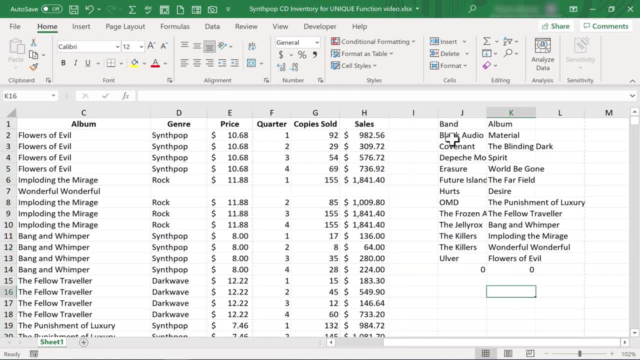 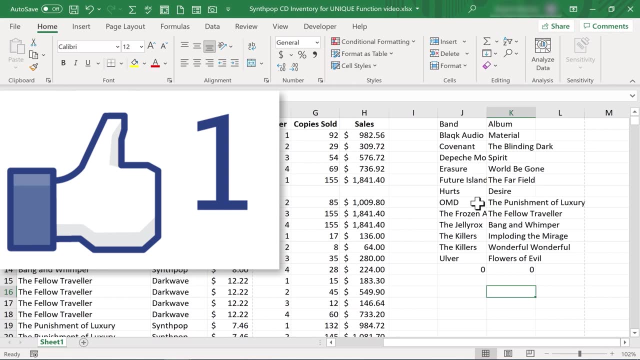 particularly exciting to do it the way I showed: To combine sort with unique in this case, but you can also combine it with other dynamic array functions to do two things at once: To produce only the unique data and then to sort it. Thanks for watching this tutorial. I hope you found it to be helpful. If you did, please. 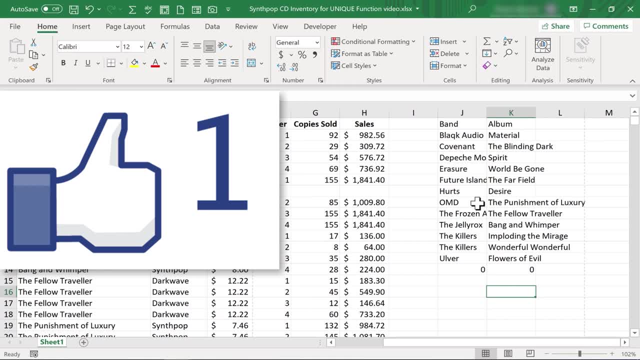 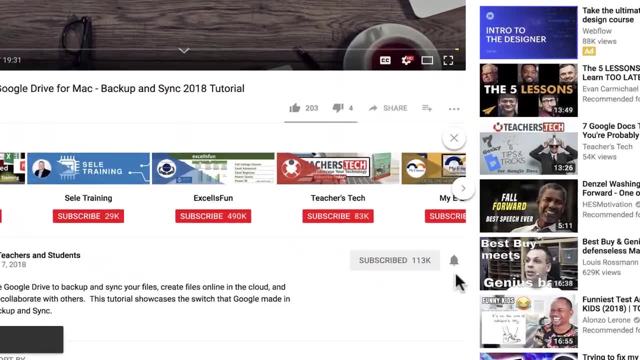 check out my other dynamic array functions videos and also my video on spilled results. But if you did find it to be helpful, please like, follow and subscribe And when you do, click the bell so you'll be notified when I post another video. If you'd like to support my channel, you can do that through my Patreon. 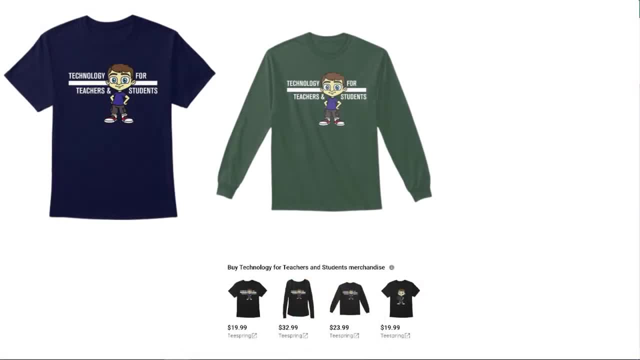 account and by buying channel merch, and you'll see links to those opportunities in the description below the video.